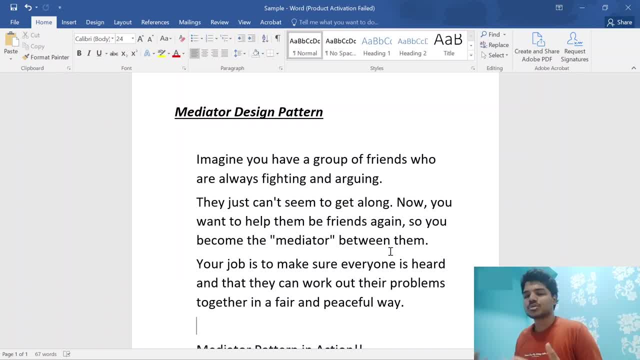 to communicate with that person, with this person. So that's exactly what mediator do, And here also, that's exactly what mediator will do In the Java also, like in a design pattern way. So this is an example of same thing. whatever I just discussed. 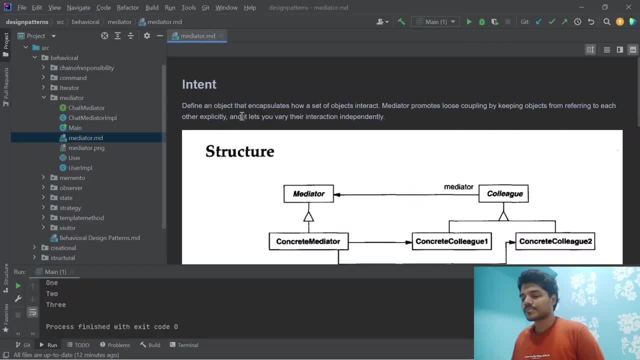 So I think no point of saying anything again. Let's see standardization. Define object: mediator: that encapsulates how set of objects interact other people Mediator promotes loose coupling by keeping objects from referring to each other explicitly. So mediator will only communicate with other people. 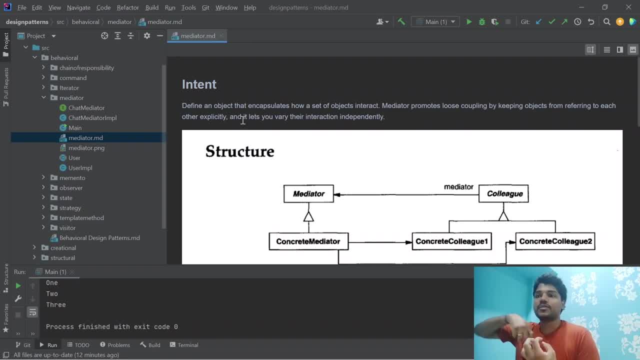 That's why it promotes loose coupling, Because if mediator is not doing like that, it becomes tight couple, Like every object will communicate with every other object. So, and also because of mediating the single person with other persons, we are reaching the single responsibility principle. 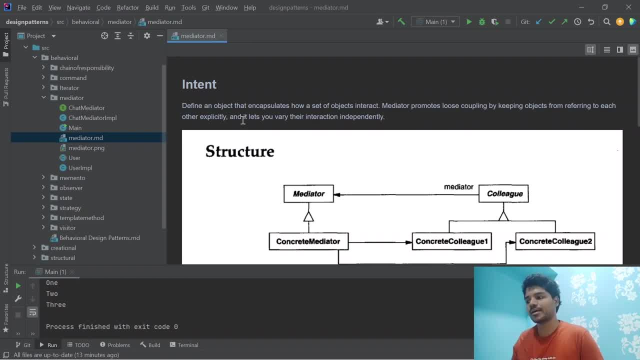 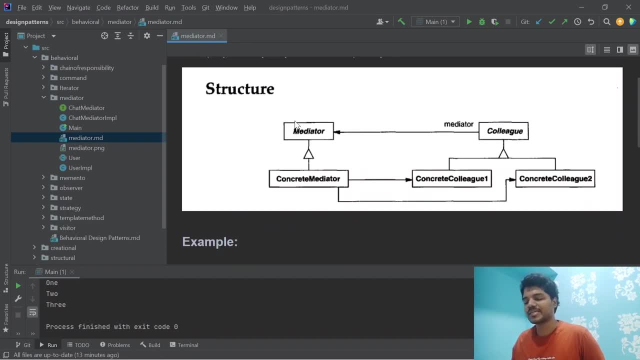 So mediator is responsible to communicate with other people And lets you vary their interactions independently. So structure is basically very simple. Like I have a mediator object, Let's say mediator interface, I have implement concrete mediator, concrete mediator implementation. So every colleague has a common friend called mediator. 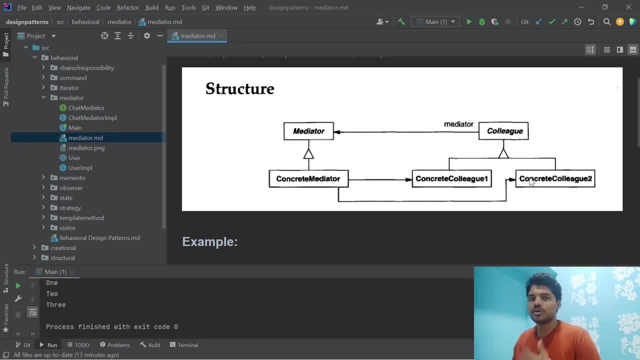 So let's say colleague 1,, colleague 2,, colleague 3.. Let's say, if you talk about like in a French language, So every colleague has a mediator. So we will just only say to the mediator, And mediator will be responsible to say to other people, all other people. 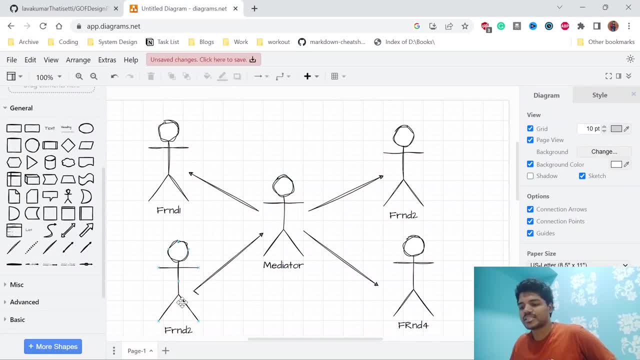 Let's see how this design looks like. So let's say, friend 2 wants to send a message to other people, But he is not talking with other people, right? He just simply sends to mediator. Mediator is responsible to send the message to the rest of the friends. 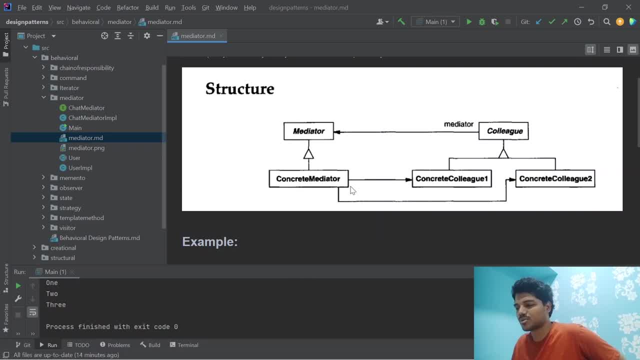 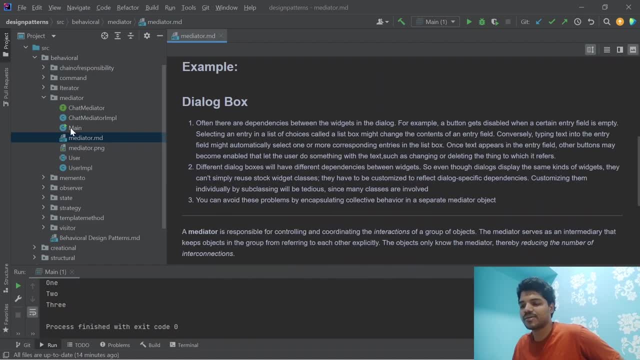 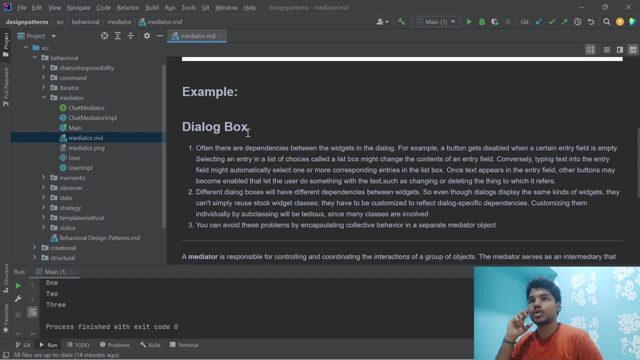 So that's how mediator program also looks like. So it's very easy thing. So before that we will just see some complex. So for complex examples then we can directly go into the Java program. Let's say: you got some UI. 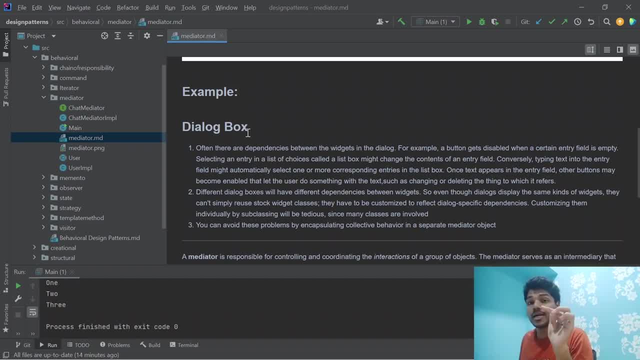 In the UI, if you see right, let's say, whenever you use a particular radio button in the below, there are some new drop downs, new fields. new fields will come, like, Let's say, initially nothing will be there. 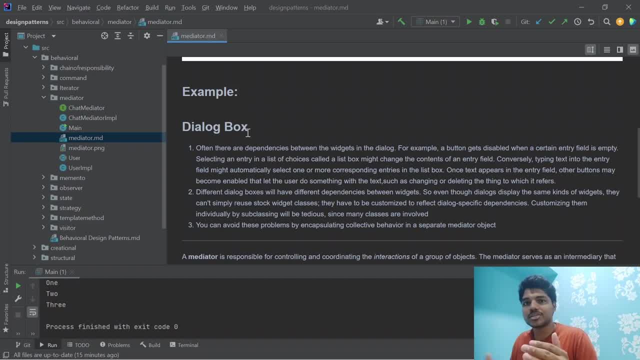 But suddenly, if you click on something, because of that action other things will be executed, And also that may not be. it can happen multiple times, also right in an application, And also when you enter a field. it might be some submit button might be disabled until. 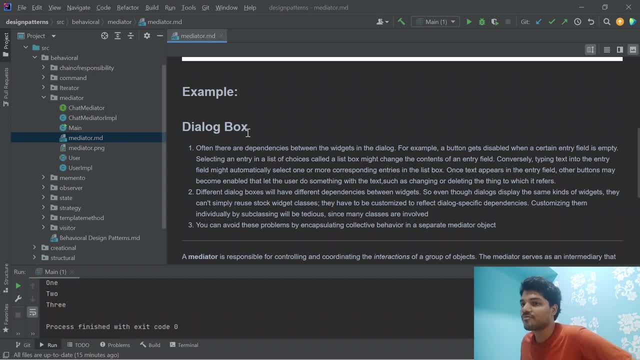 unless you enter all the fields, So you will see all the validations right that we can correlate it as a mediator. like So often, there are dependencies between the widgets in the dialog. For example, a button gets disabled when a certain entry field is empty. 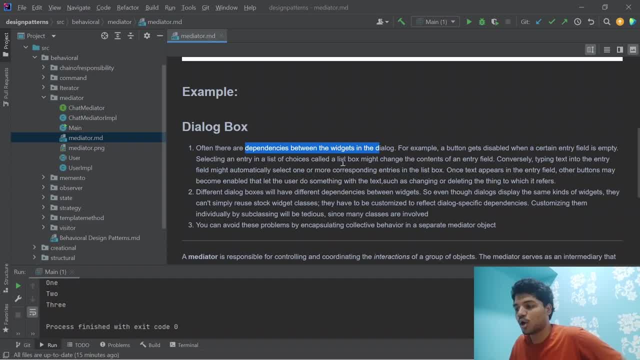 So selecting an entry in a list of charges called a list of charges. So that's how it works. A list of charges, called a list box, might change the contents of an entry field. So, conversely, typing text in the entry field might automatically selects one or more corresponding. 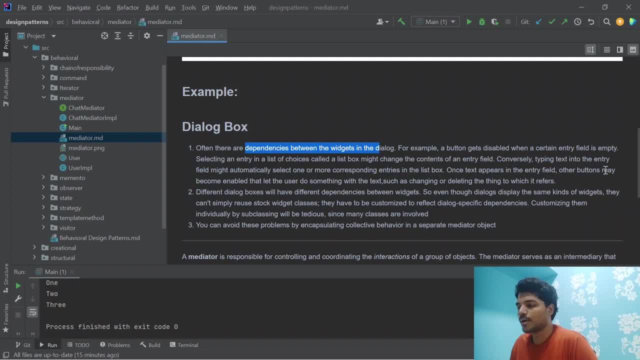 entries in the list box. So buttons may become enable or disable. So different dialog boxes will have different dependencies between widgets. So even though dialogs display the same kind of widgets, they can't simply reuse log widget classes, So they have to customize it to reflect dialog specific dependencies. 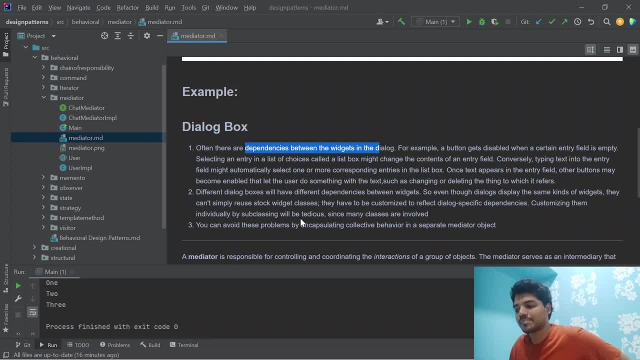 So customizing them individually by subclassing will be tedious, So we are basically changing it at a single point. It will be that one basically helping us to communicate with others like. So you can avoid this problem by encapsulating a collective behavior in a separate mediator. object: 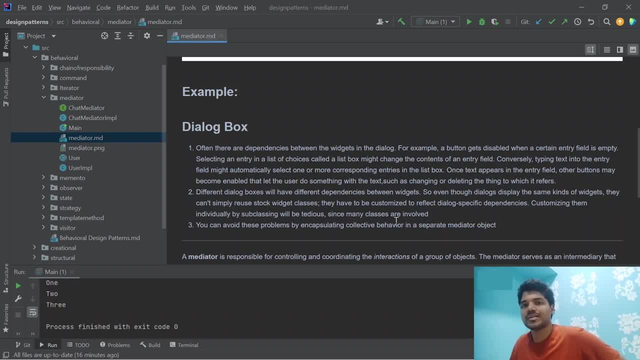 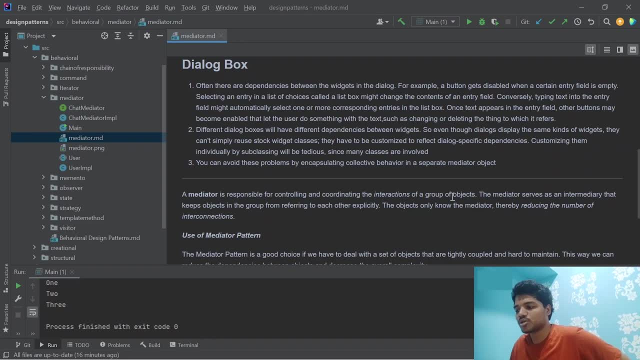 So you are doing all these things in a single object and let people communicate with others how others should respond like. So a mediator is responsible for controlling and coordinating the object And coordinating the interactions of group of objects. A mediator serves as intermediary that keeps objects in a group from referring to each other explicitly. like 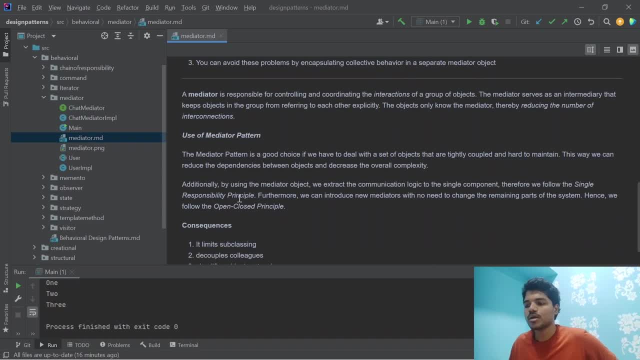 Thereby reducing the number of interconnections. Use the mediator design pattern is a good choice when you don't want tight coupling, when you want to provide a loose coupling, Because tight coupling is ultimately hard to maintain, And also it will also follow single responsibility principle we just now discussed. 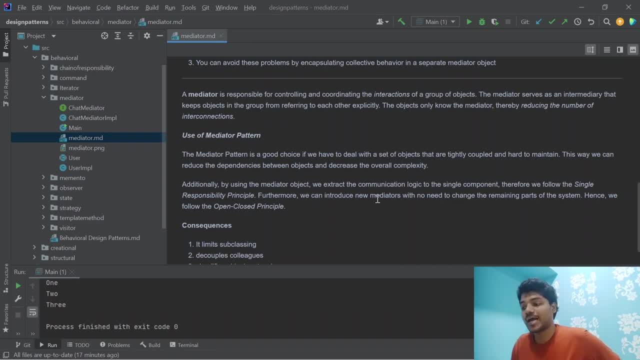 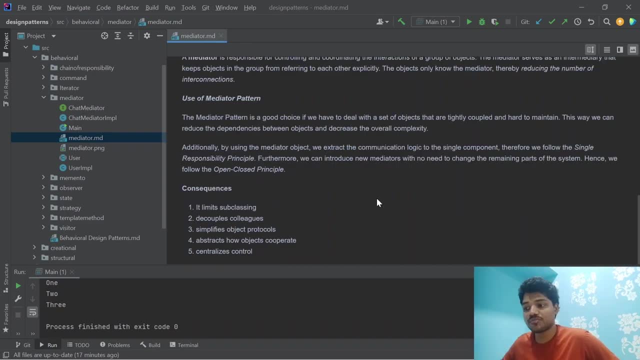 And we can introduce as many mediators without changing the existing behavior, like Open for extensions, adding new mediators and close for modification, Modification of the existing one. Use of mediator pattern is a good choice if you are dealing with a set of objects that are tightly coupled and hard to maintain. 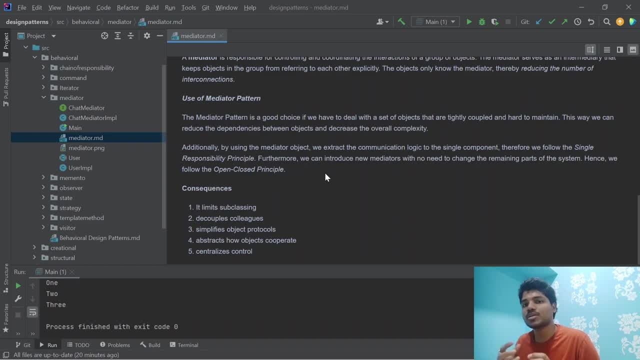 And also, if you want, to reduce the dependencies between the object communication And by using the mediator pattern. we are like providing single responsibility principle, And there can be many. number of mediators can be added without basically breaking the system, Which will also following the open-close principle. 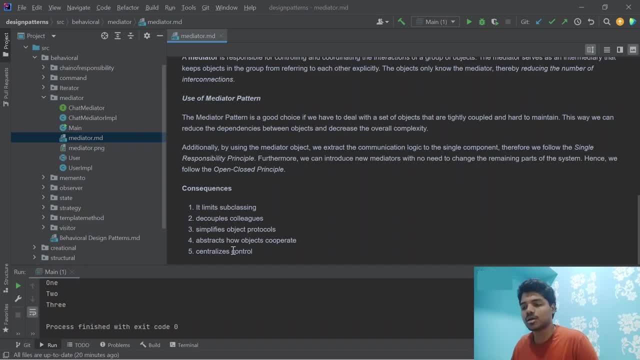 So there are, like some of the advantages, basically Centralized control, Abstracts how objects cooperate, Simplified objects, protocol, Decoupled colleagues And limit subclassing. Centralized means it's like mediator- is only one, communicates to others right. 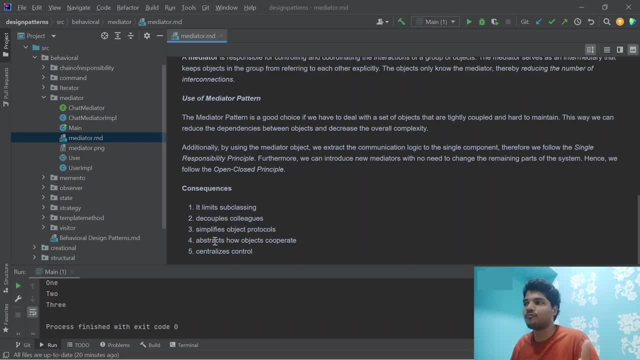 And abstracts how objects cooperate. One object how it will operate, other objects It don't know, like Like, mediator is responsible. So thereby this protocol is also simplified. Like when you want to communicate with another object, It will directly communicate with the mediator, right? 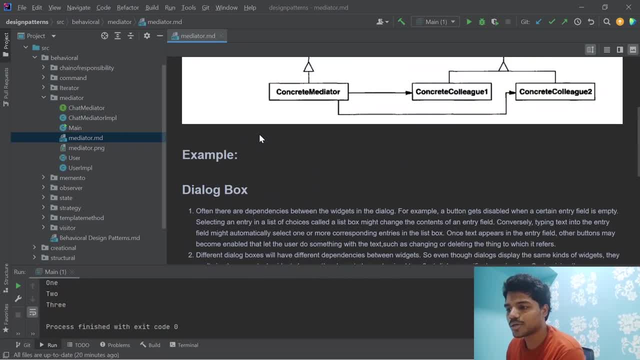 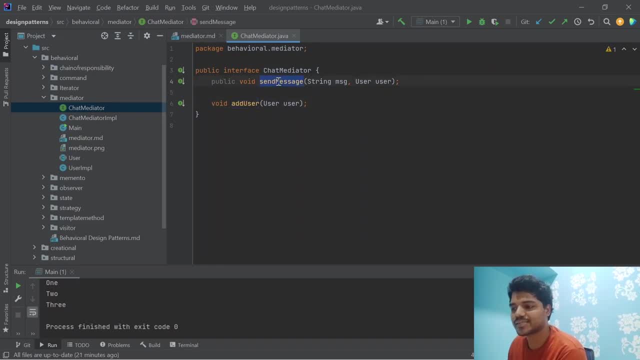 Let's see an example to get a better idea. So here, according to the class diagram, We have a mediator called chart mediator. It has two functions: One is like add user And second thing is like send message. So add user is basically adding the users. 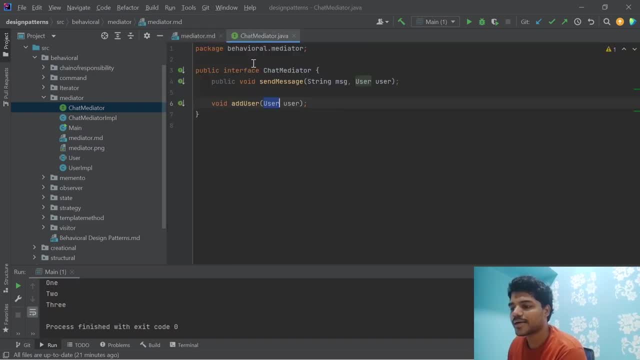 Which is nothing but adding. a colleague like And message is basically sending a particular message, So this user is basically sending this message. So we have chart mediator, IMPL, So we have send message right. So this user is sending this message right. 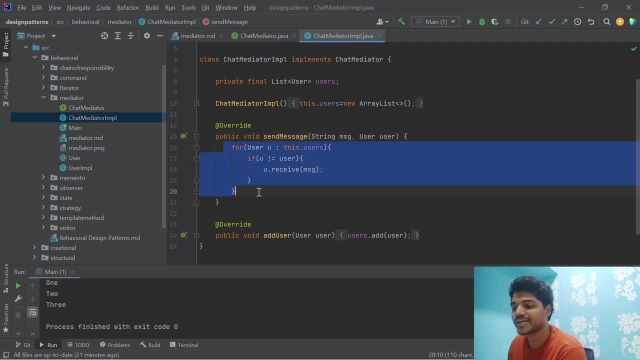 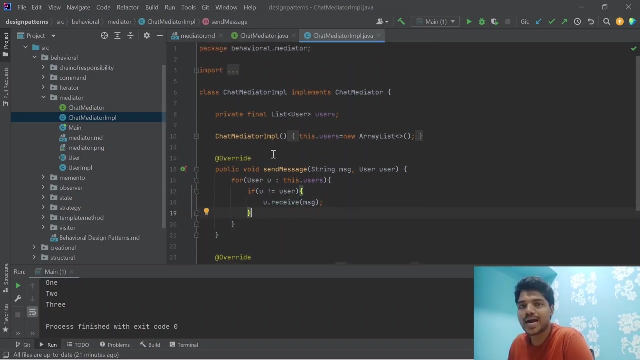 So as mediator is central point of communication, So mediator is responsible to send the messages to all the other messages To all the other users, right? So, from mediator, every user will get the message And if you want to add the users into your group, 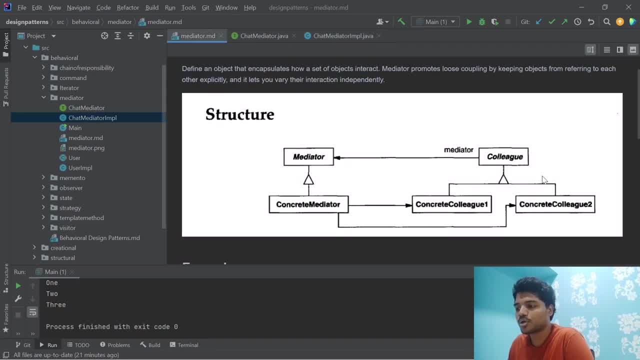 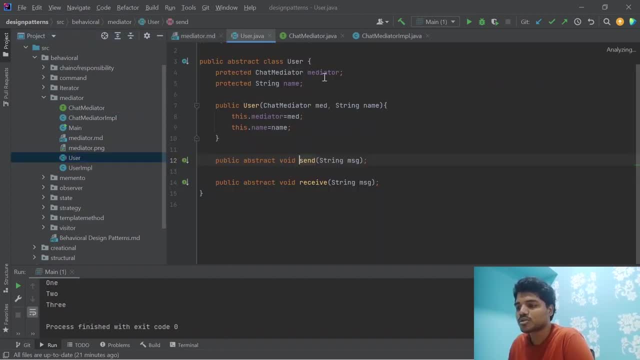 Through mediator you can add the users. So according to the diagram, So colleague has a mediator, right In our classes. colleague is basically user. So user has basically mediator And user has already name. So it has like constructor called like mediator. 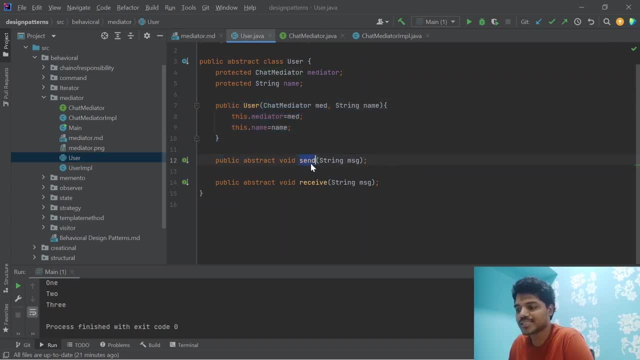 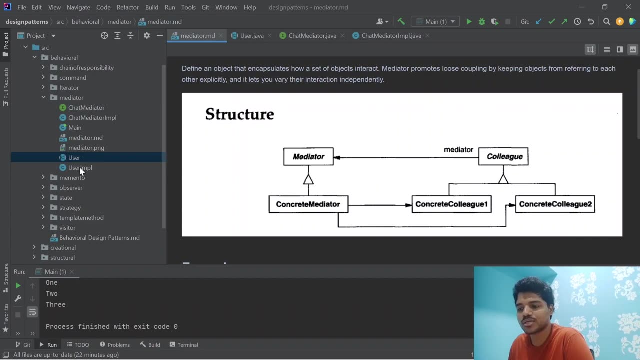 And also name. So it has like two functions. One is like send, Second thing is like receive, So it has like concrete colleagues are there. For now I have created only user, Only one user like. So user has like user message. 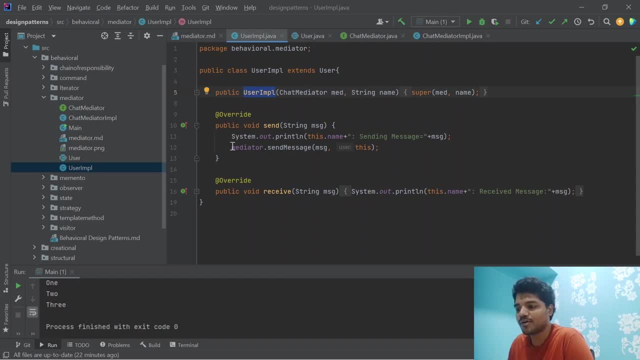 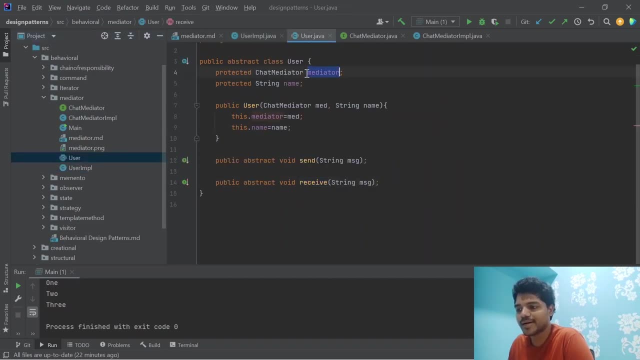 Like user. IMPL has like mediator name. So here first is like: whenever sending Through mediator, we basically send message. So anyway, that user has like mediator, right, We are using that mediator to send the message. like To send the message. 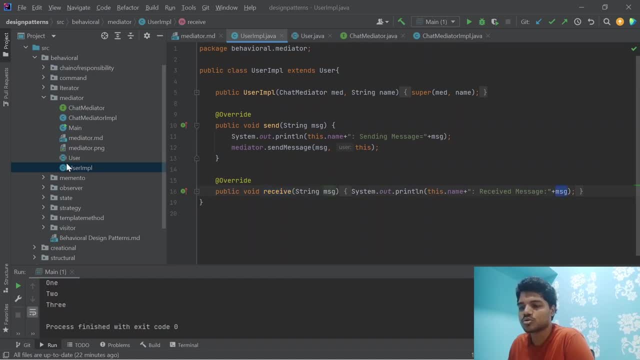 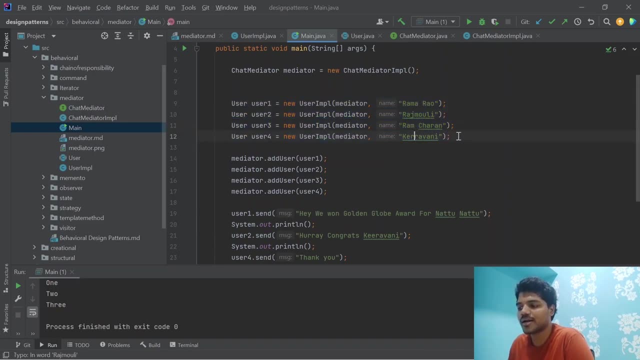 And whenever receiving we just getting the message like: So in the main program We have like around four users are there, Let's say Ramarao, Rajamouli, Ramchand and K Ramani. They are like RRR crew. 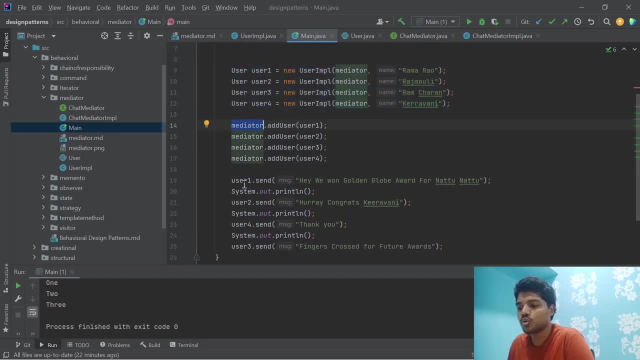 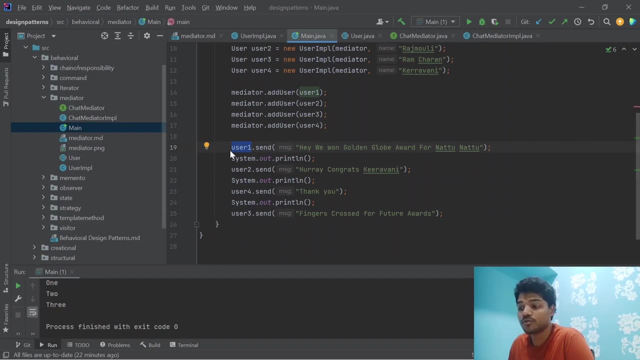 And we are adding all the users into the mediator. Now user one sends the message: Hey, we won the golden globe award for Naatu Naatu. So, and also, if user one sends, like when Ramarao sends the message- Rajamouli, Ramchand K Ramani will get. 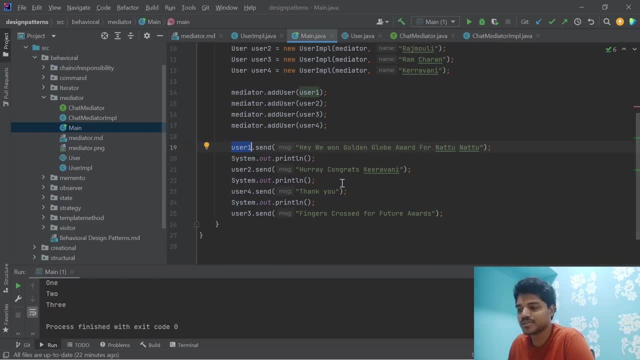 When user two sends message like congratulations, like, And also user four sends the message thank you, And Ramchand is saying for fingers crossed for future awards. When you execute this one right, You will understand how the communication happens like. So first Ramarao sends the message. 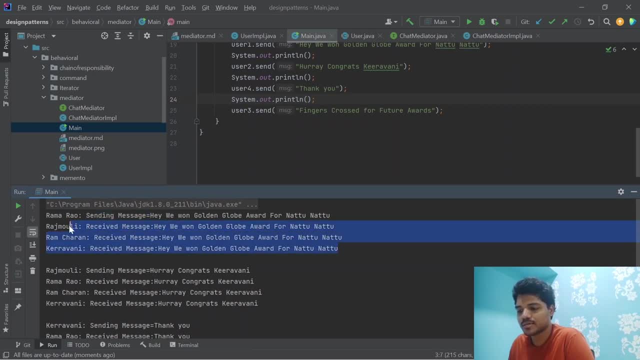 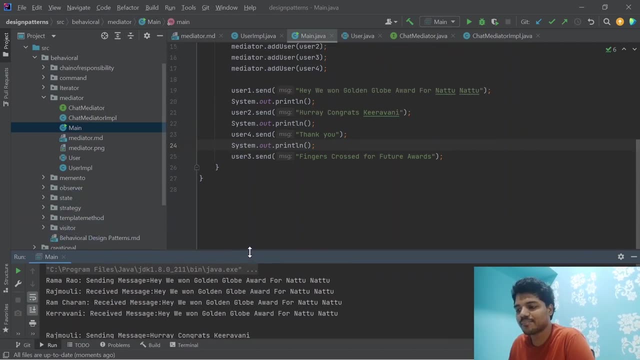 And Rajamouli, Ramchand and K Ramani receives the message. Similarly, Rajamouli sends the message And Ramarao, Ramchand and K Ramani receives the message. Likewise, one is basically sending the message to the mediator. 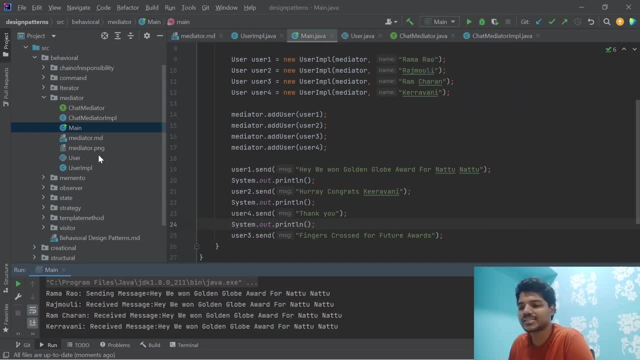 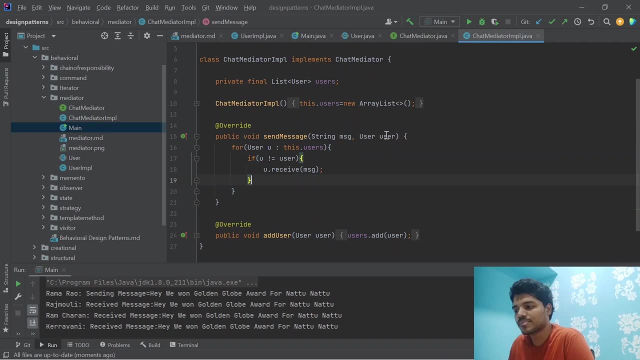 Mediator is basically sending the messages to the other people like: So in the mediator IMPL we have like all the users. So from this user, mediator is basically sending the messages like: So all the users are basically receiving. So this is how a simple mediator we can implement with the help of Java. 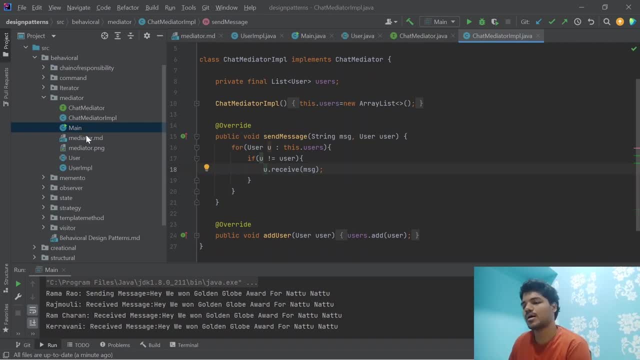 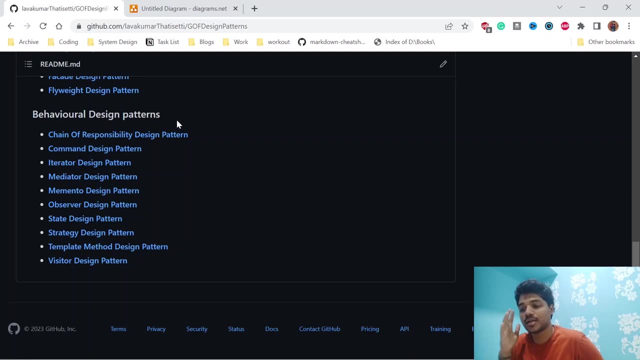 And mediator is also one more easy design pattern. So I think that's it for today's tutorial. I hope you got what exactly mediator design pattern. If you have any doubts, please your comments in the description In the comment box. I will try to reply most of the comments. 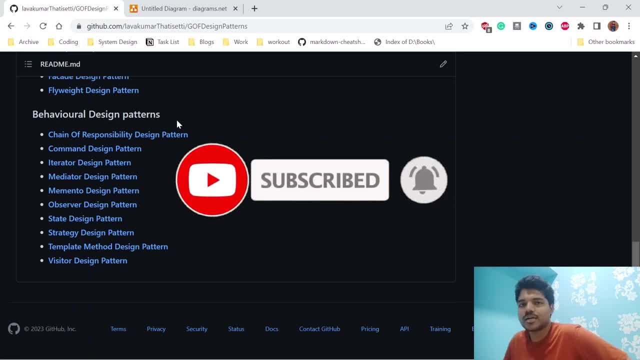 If you like the video, please subscribe and like And share to your friends also So that they can also get benefited. like In the next video we will discuss about: like memento design pattern. like So soon we are completing the behavioral design patterns. So for now bye, bye.